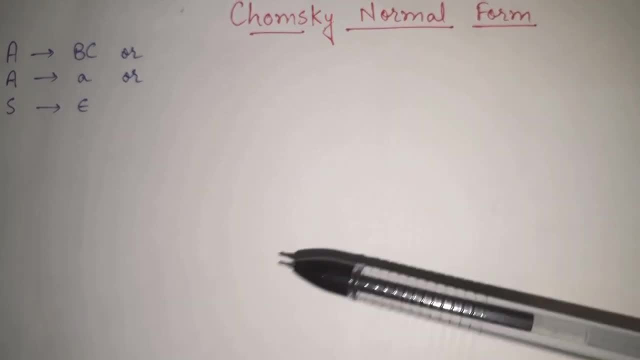 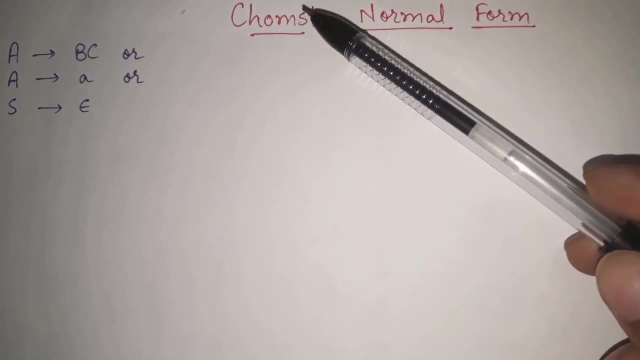 are the different types of grammar right? What are the different categories in which the context-free grammar can be categorized? We will also see that Now. first of all, we should know that what is Chomsky normal form? So any context-free grammar can be. 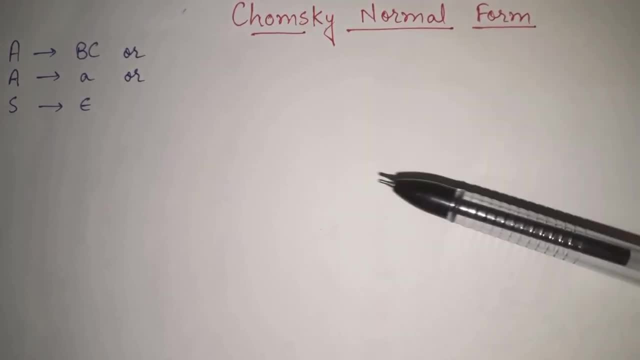 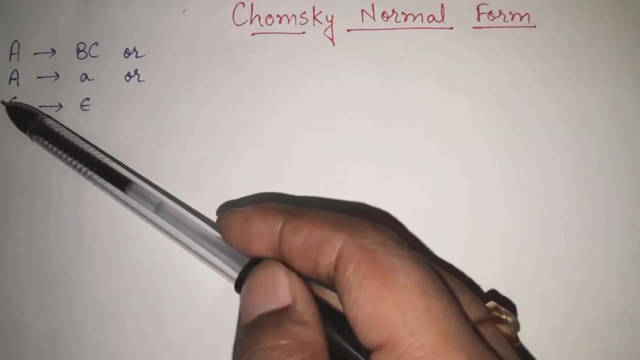 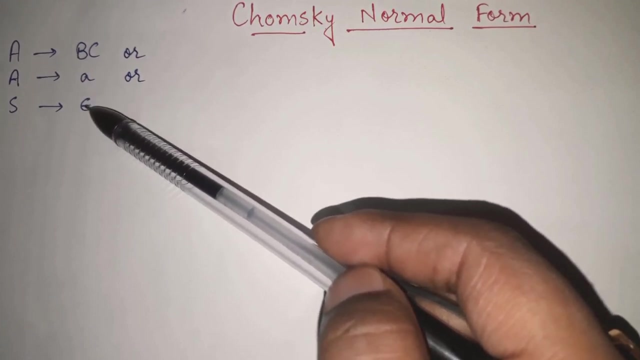 said to be in Chomsky normal form, if all of its productions are in any of these forms, which are the main forms: A gives BC, A gives small, a S gives null. where S is my starting symbol, this epsilon is my null production. null means nothing: capital A, capital B. 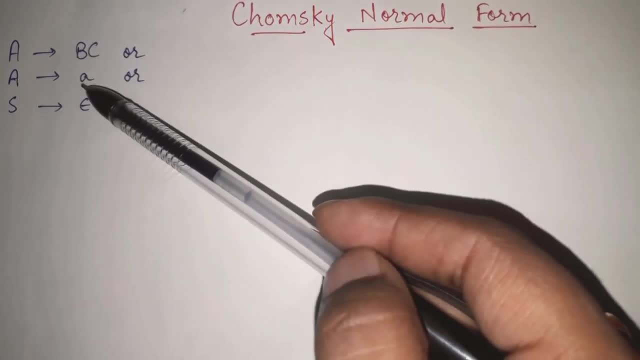 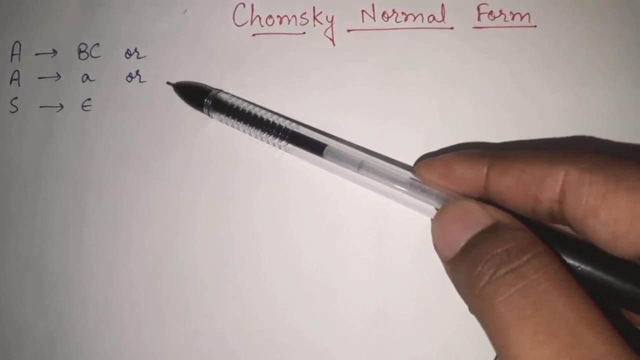 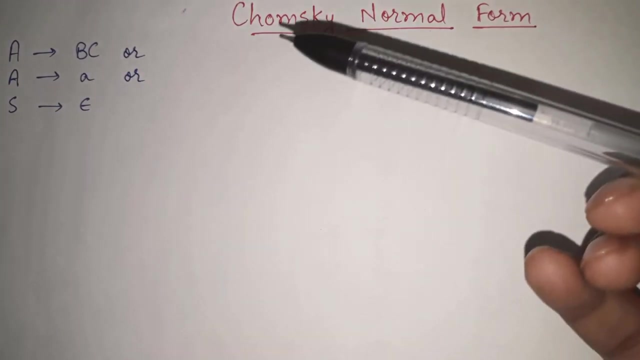 capital C are my non-terminals or variables, And this small a is my terminal. So if all the productions present in my grammar is in any of these forms, I can say that my that is CFG, or that context-free grammar is in the form of Chomsky normal form. Fine, this is the basic definition of Chomsky normal. 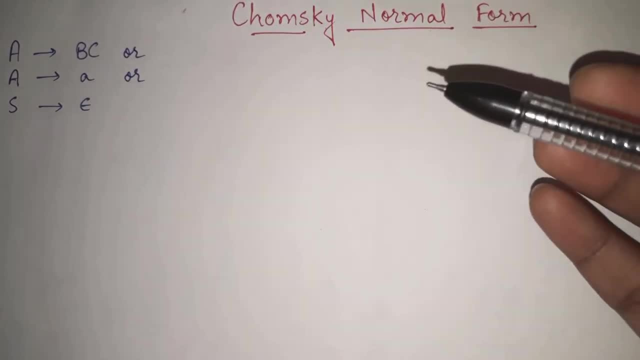 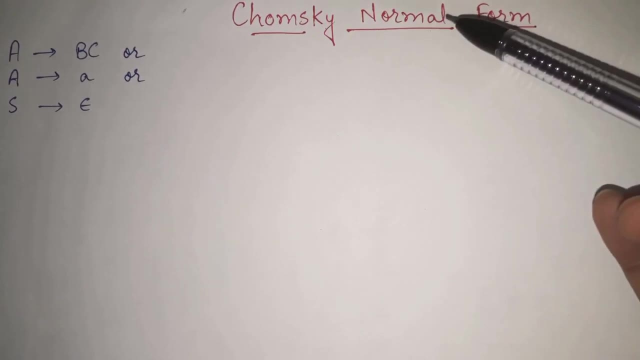 form. Now the main thing to be understand. one of the important things here to understand is which are the different types of grammar that are categorized as per this Chomsky normal. So let's go into that Chomsky normal form as per the hierarchy of the Chomsky normal. 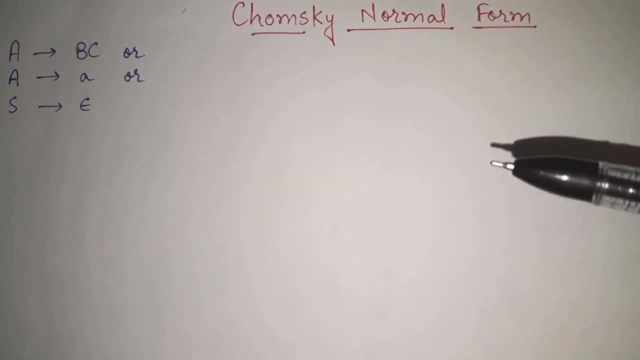 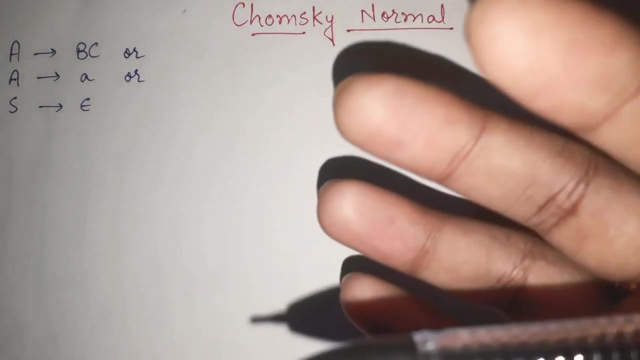 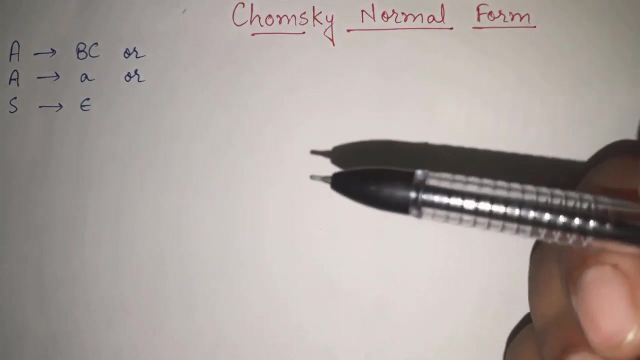 form, our CFG or any context free. grammar can be categorized into four main parts. these four types of grammar are actually very important in case of academics in like BTech, MTech, or in case of any competitive exams like GATE, ISRO, ONGC, etc. this is a very popular topic. 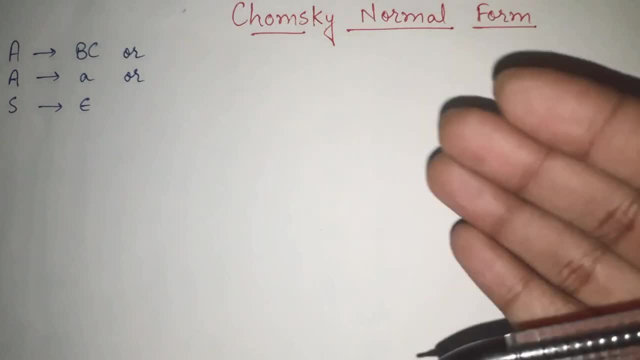 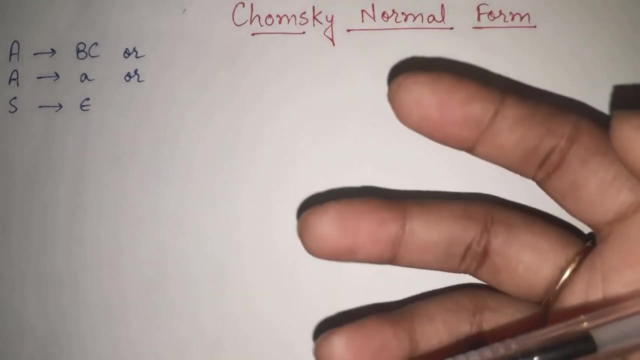 that is being asked in various interviews also, that which are the different types of grammar and based on those grammars, various things can be derived, various questions can be asked. So let us understand this in the basis of this Chomsky normal form or hierarchy of Chomsky. 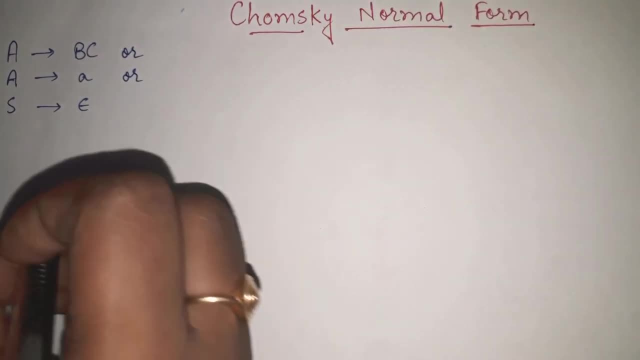 we can say that our types of grammar are categorized into four. these four categories of grammar are type 0, type 1. this is very important to remember Which are the grammars and what are the specifications. type 0, type 1, type 2, type 3. these are the 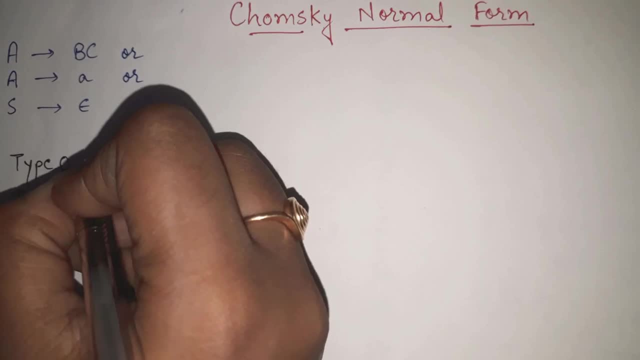 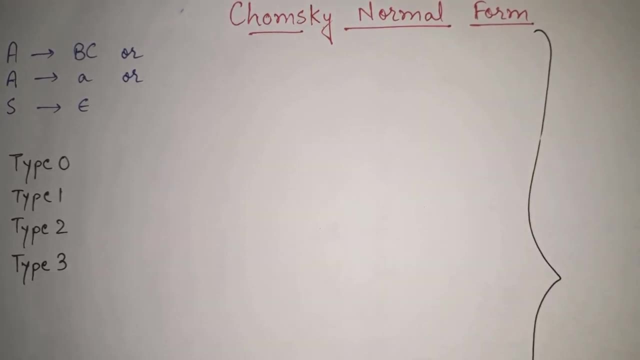 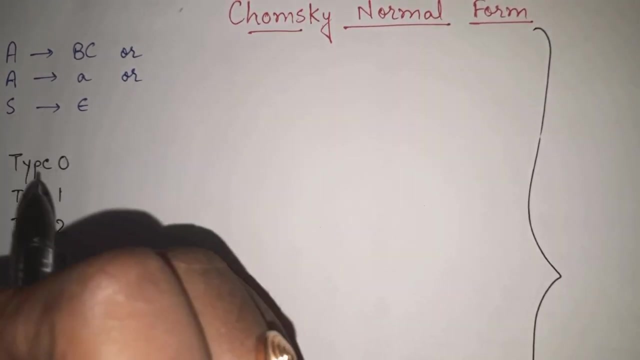 main four types of grammar. now, what are the things that you should be remembering? let me categorize here which are the different things that you should be remembering: that what is the name of the grammar, by which the grammar is denoted, and what is the machine that can identify that grammar. fine, these are the frequently asked questions that you 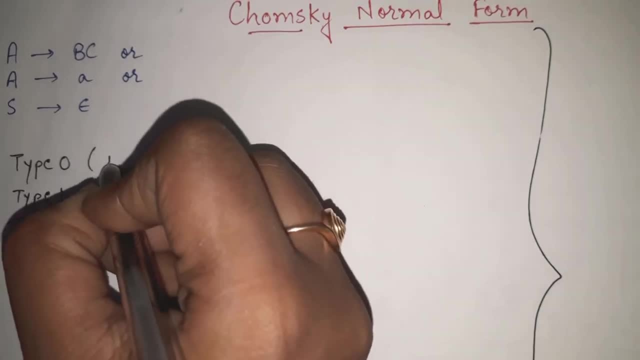 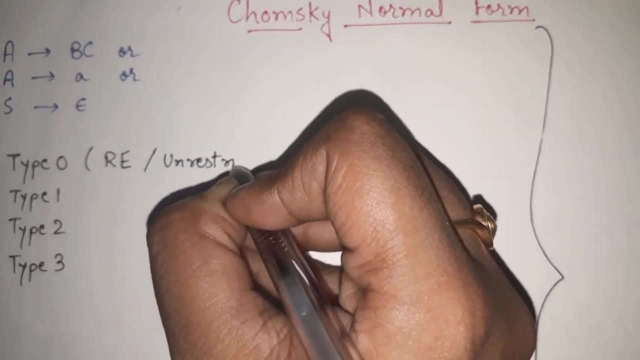 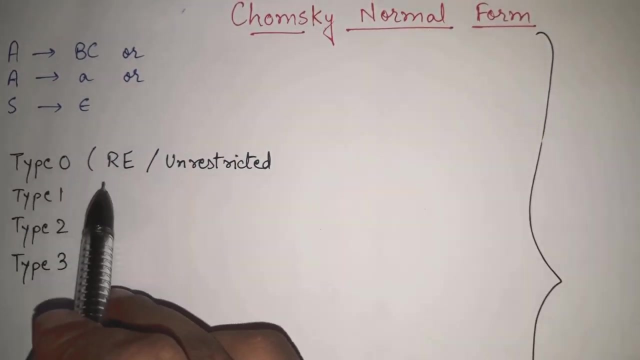 must be knowing. So type 0 grammar is also known as recursively enumerable grammar or unrestricted grammar. the name is same for the grammar or language. fine, so this type of grammar is known as recursively enumerable grammar or unrestricted grammar, or such languages. are you understand that? 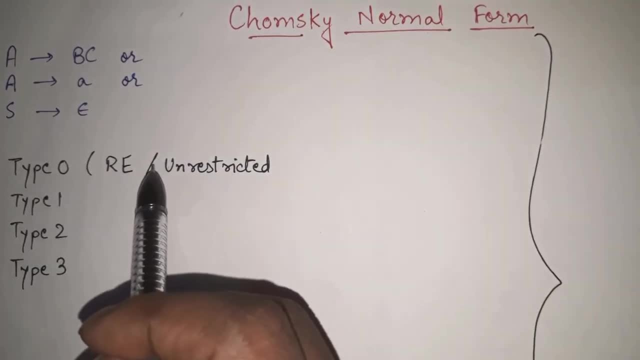 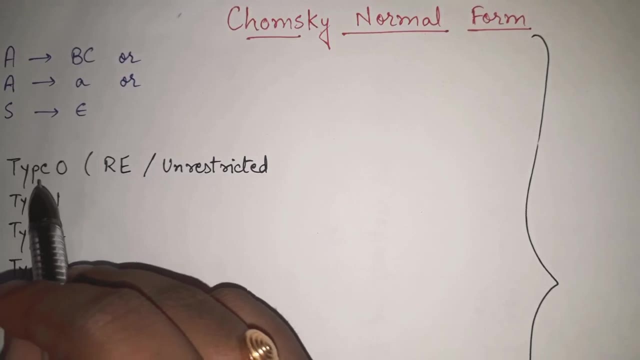 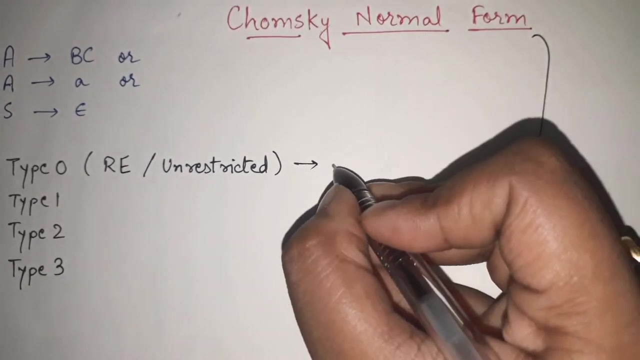 internally right if I tell this. the grammars are also named like this, like recursively enumerable grammar, And languages also that recursively enumerable language or restricted language. so in short, type 0 is recursively enumerable or restricted, and the machine that can recognize this is known as Turing machine. 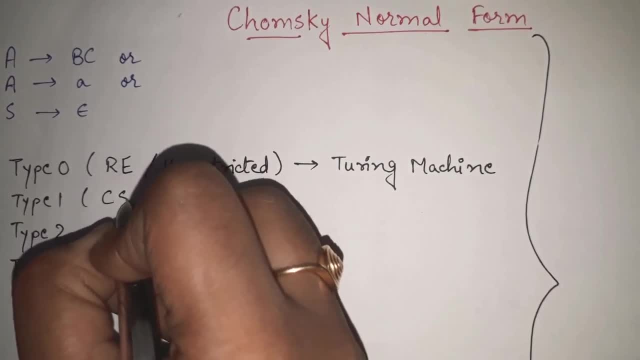 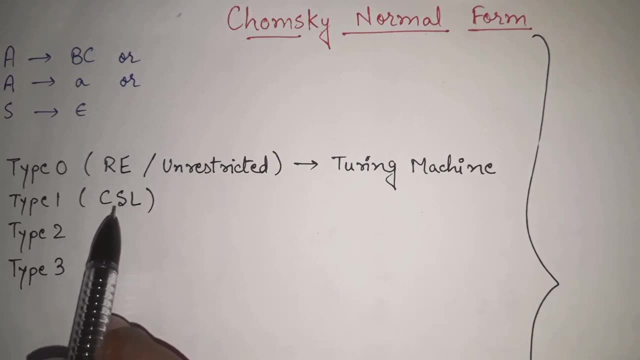 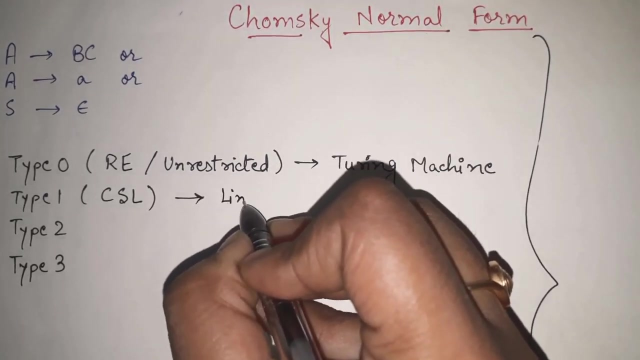 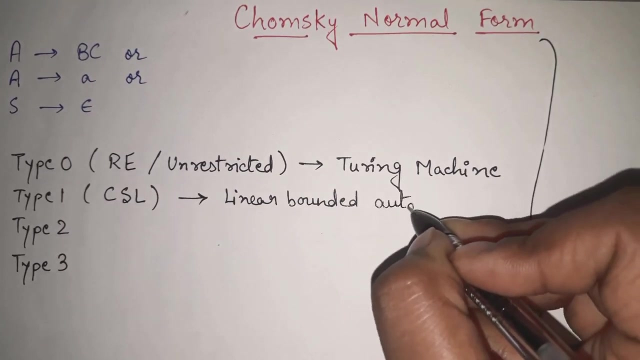 What is type 1,? type 1 is known as context sensitive language. the languages of type 1 are context sensitive language and the grammar respective grammar is known as context sensitive grammar, and the machine to recognize this type of grammar is known as linear bounded automata. fine. 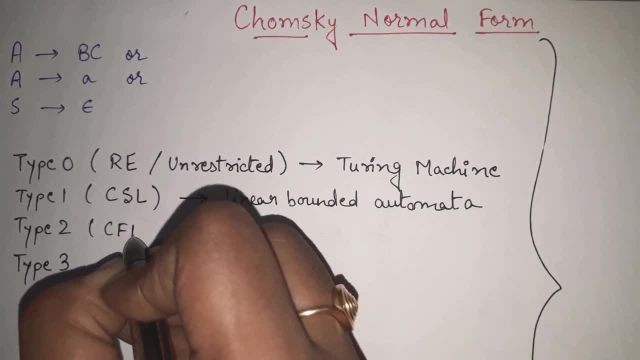 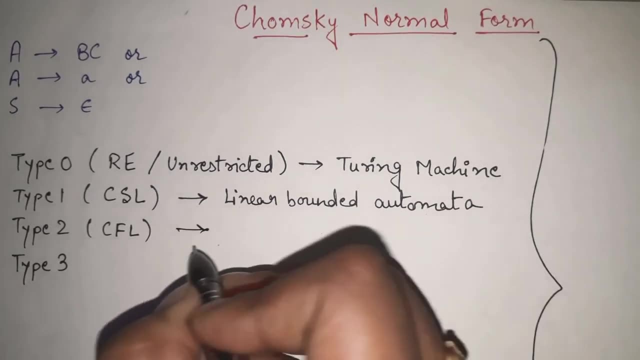 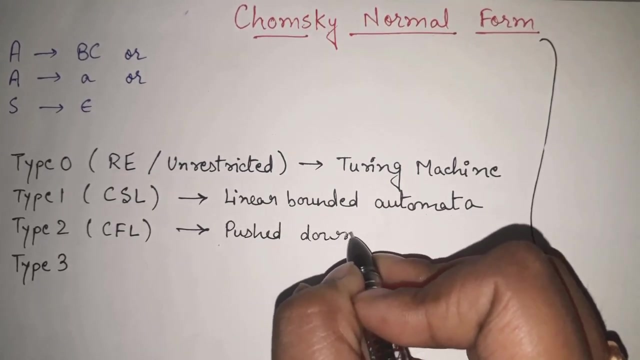 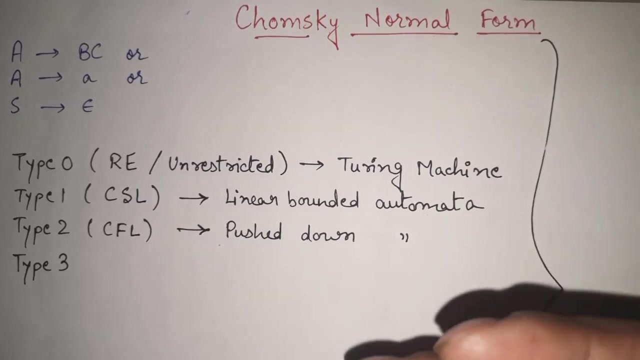 If I talk about type 2, it is known as the languages are known as context free language, and the grammar respective grammar is known as context free grammar and the machine that is used to recognize this is known as pushed down automata. Thank you, In our respective videos we will see these also in detail, but the aim of this video is 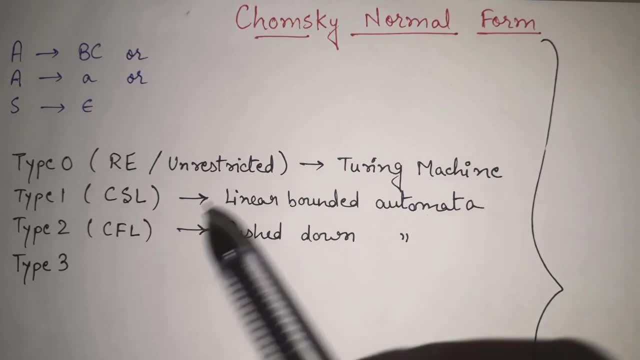 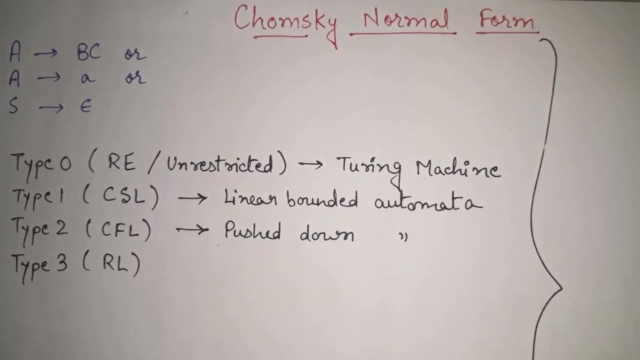 to understand the difference between these four grammars. right, it is important. So type 2 is context free language. the respective grammar would be context free grammar, and the machine that is used to recognize this type 2 grammar is pushed down automata. Now type 3- the languages of type 3 are known as regular language, the respective grammar 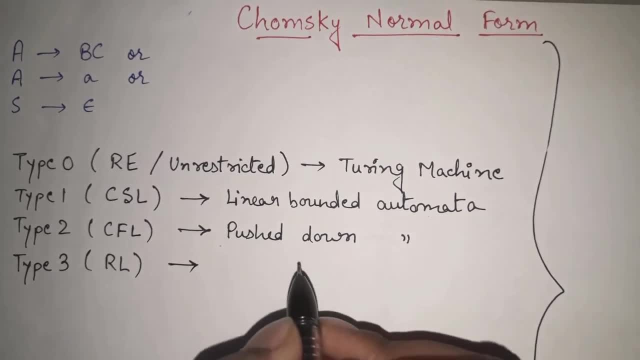 will be known as regular grammar, and the machine that is used to recognize this type 3, it is known as finite automata. it is again of two types: determinant finite automata and non-determinant finite automata. it is in case of these also that we are having in PDA push. 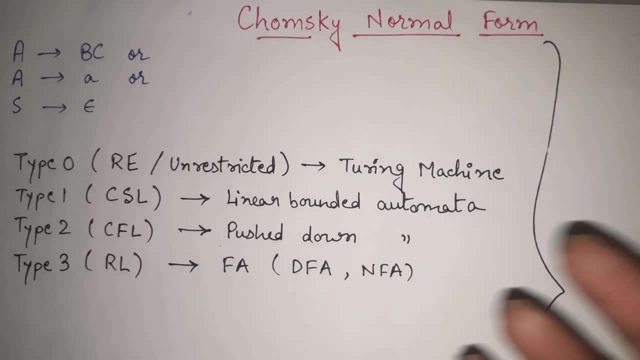 down automata. also, we are having deterministic and non-deterministic, So, however, we will discuss about that later, but these are the things that you should be remembering: the machines and the types of languages that we are having for these four grammars. fine, this is one of the important things to remember now. apart from this, the 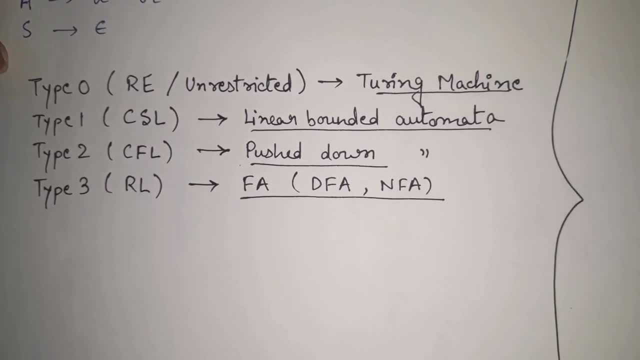 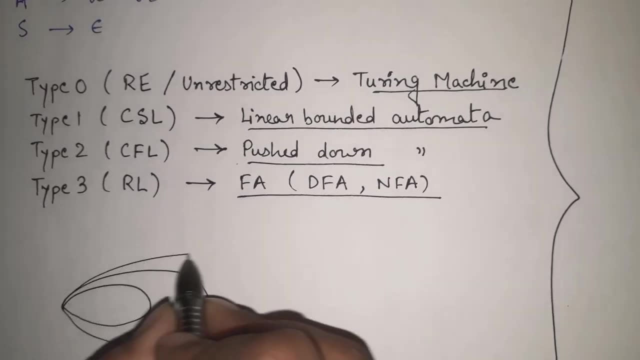 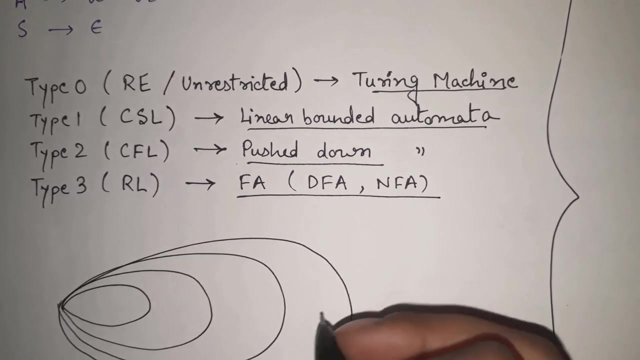 main hierarchy that you have to remember is: I have already told you about these grammar. now we are having hierarchy like this. hierarchy means the relation between these four grammars, the type 0 grammar. it is our unrestricted grammar. as the name itself indicates, it is unrestricted. 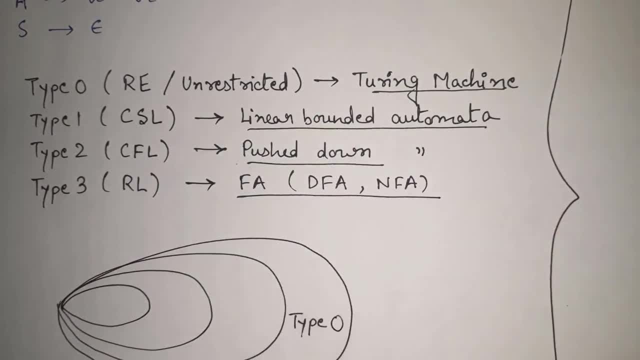 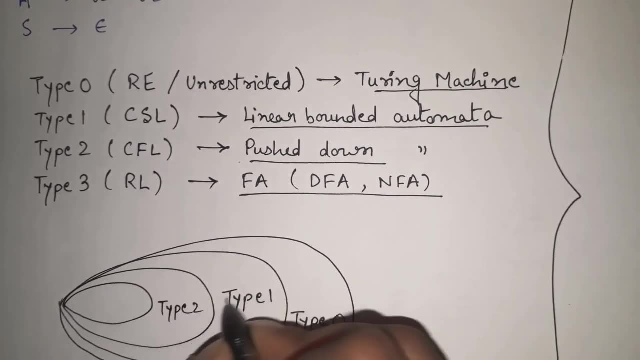 There is no restriction in that grammar. so it is the biggest form of grammar. here I will be having type 1, here we will be having type 2 and innermost we will be having type 3.. So what are you understanding from this hierarchy? that my any grammar, if my any grammar, is type. 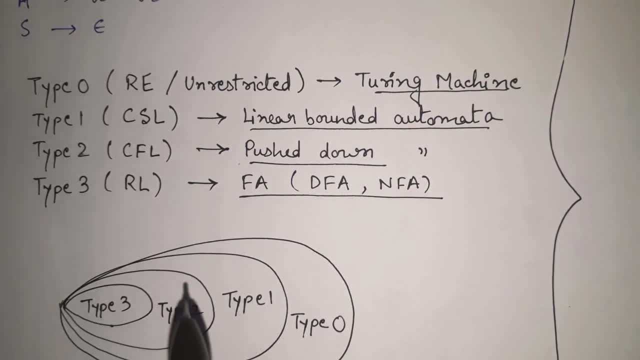 3, I can say that it is automatically type 2 and type 1 also. fine. similarly, if my any grammar is type 2.. I can directly say that it is type 1 and type 0 also. similarly, if my any grammar is type 1, it is by default type 0.. 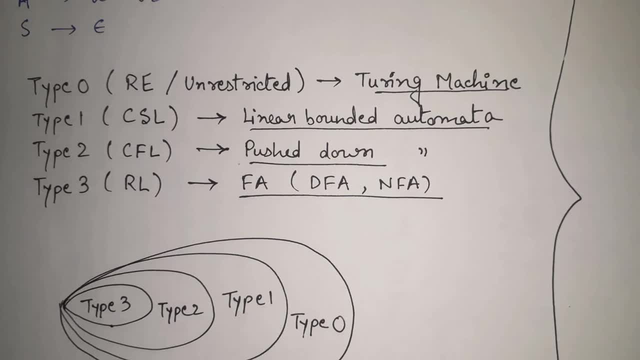 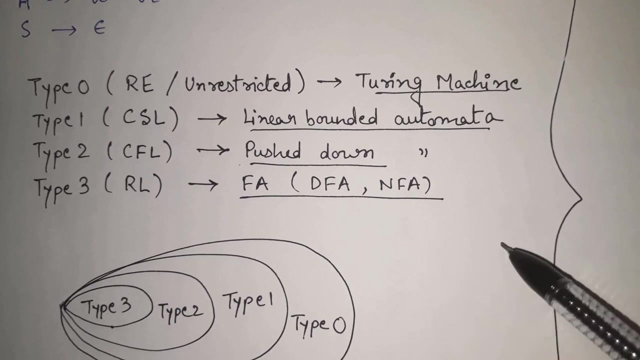 So this is one of the important things that you should know so that it can help you simplify many questions. fine, so you should remember this relation between the grammars. ok, now the mostly asked questions are similar. like they will give you a grammar and, based on the grammar, you have to tell that what is the type of this grammar? 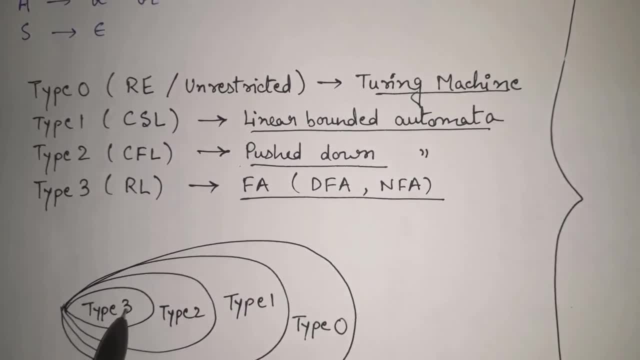 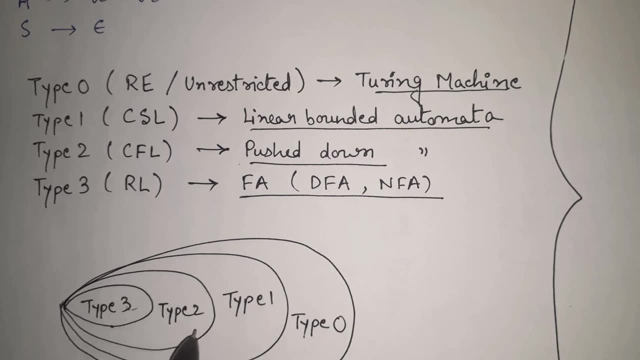 Ok, Fine, again, remember this thing that if any grammar is type 3, it will automatically be type 0, 1, 2. if it is type 2, if I know that any grammar is type 2, it will by default be 0 and 1 also, and if I know that any grammar is type 1, then it is automatically be type. 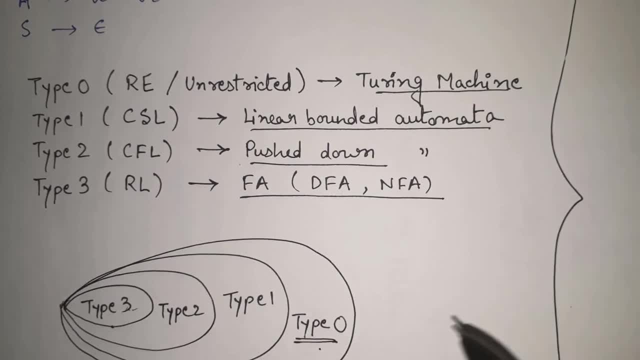 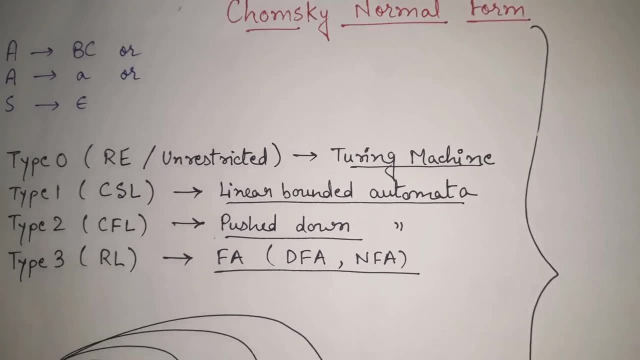 0 also, and type type 0 is the most unrestricted grammar. and now let us see that if any grammar is given to you and you are asked to specify that which type of grammar is it is now, then at that case, How will you specify, or how we can identify that what is the type of grammar? so see I. 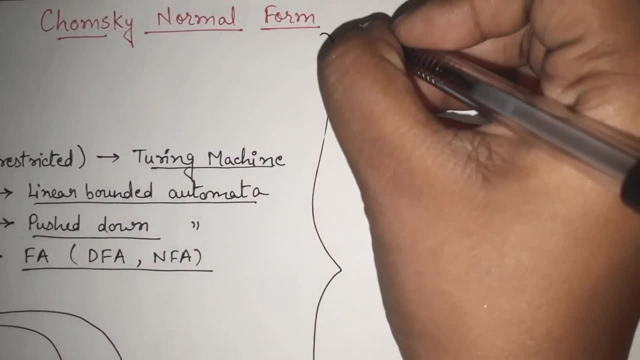 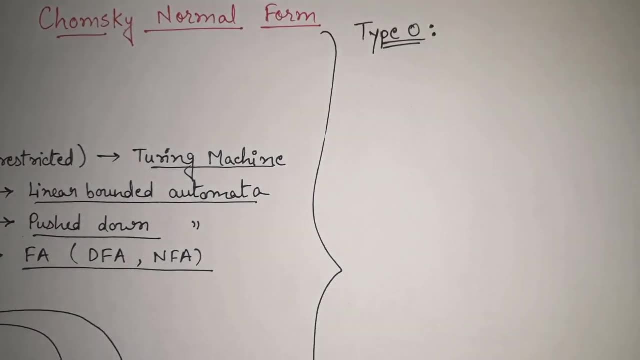 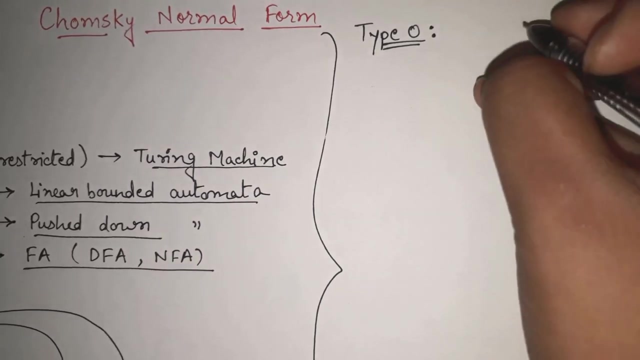 am telling you the specification, how we can understand. first of all, what about type 0? as I told you, type 0 is the most unrestricted grammar, so that means what the least number of restrictions will be in this type 0. so we are taking, see, let us, let me tell you something. 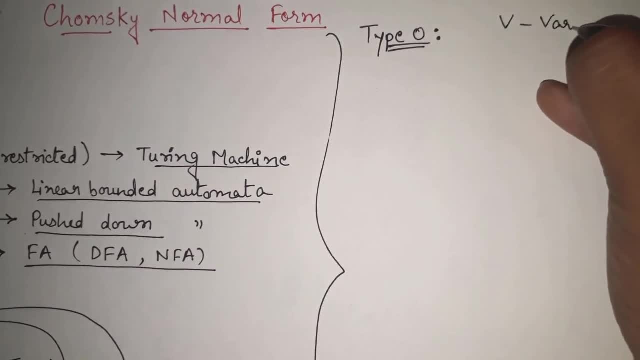 in all this, I will write. I will write v for variables. what is variables? variables are also known as non terminals. I will write t for terminals, t for terminals, v for non terminals, because non terminals are also known as variables. so t is terminals, non terminals or variables is v. epsilon is. 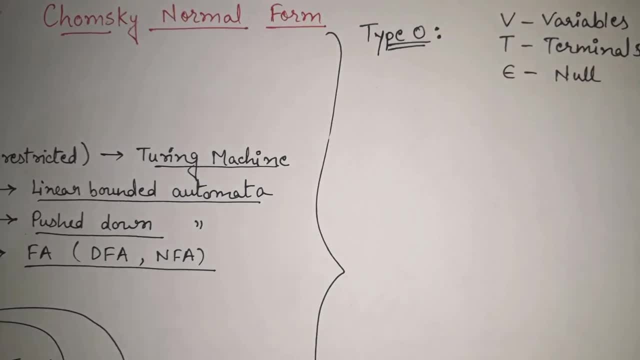 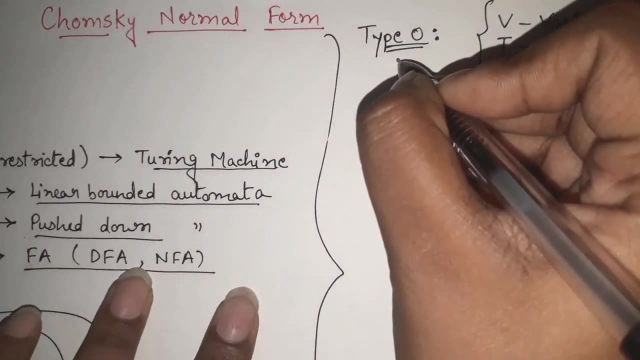 for null. fine now, first of all, this is general right for all types of grammar. now, if I talk specifically for type 0. How we can, How we can, how I can say that my any grammar is type 0 or not. for example, I am having grammar. 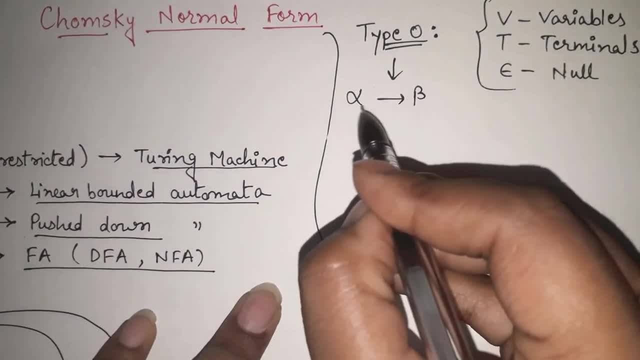 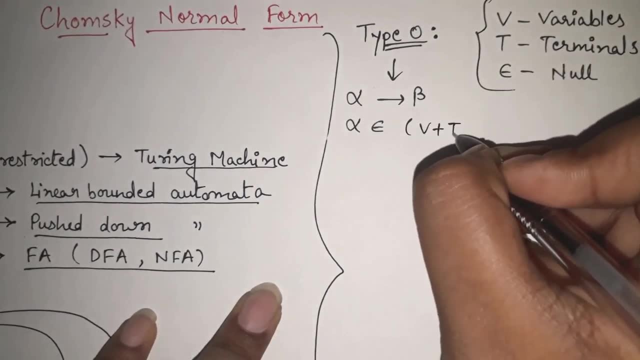 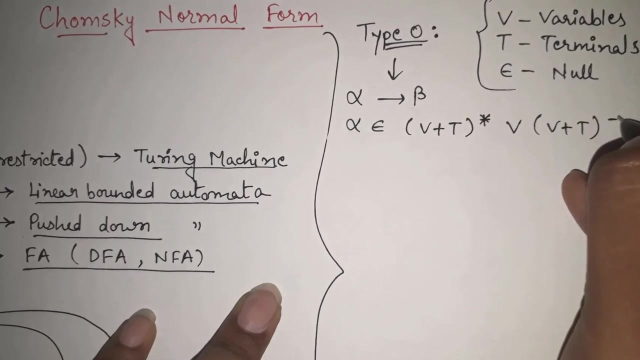 alpha gives beta. in this case I can say that my this grammar is type 0. for that the only condition is: alpha should belong to v or t star when v is compulsory, and then again v plus t star. and about beta: alpha means this one, beta means this one, and for beta I am. 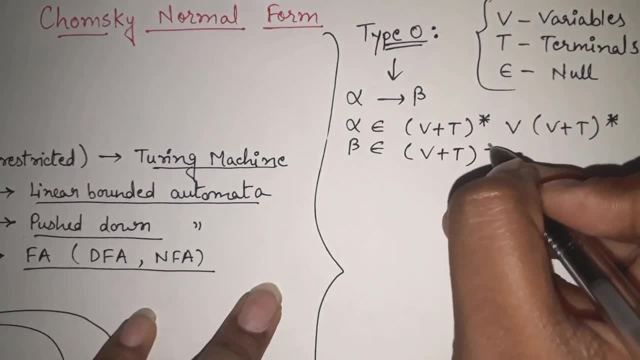 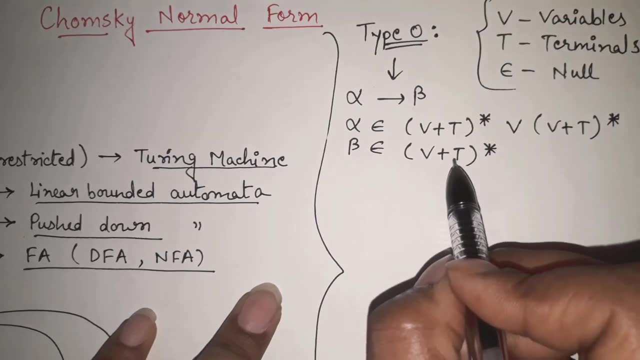 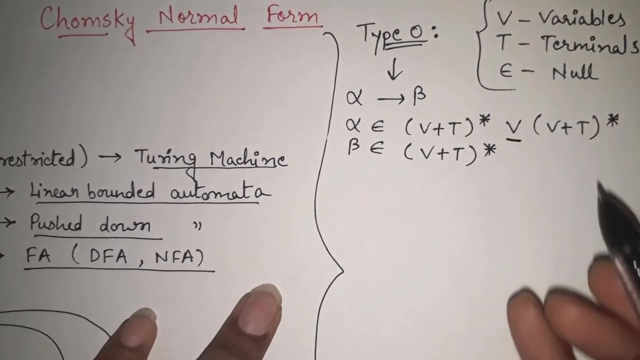 having no restrictions. beta can be anything, either variable or terminal or null. what is this? v plus t star means it can be either variable or terminal or null. and what about alpha? the only condition about alpha is alpha is having one variable compulsory. it can have either variable or terminal, or 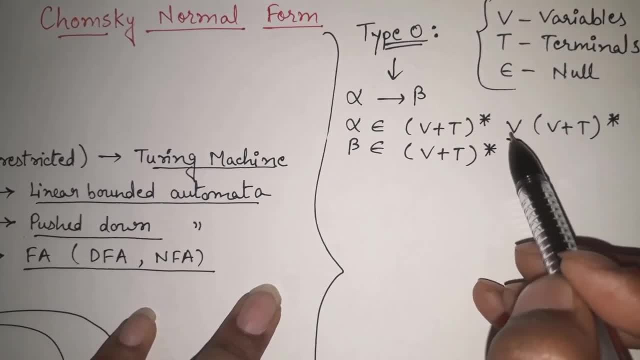 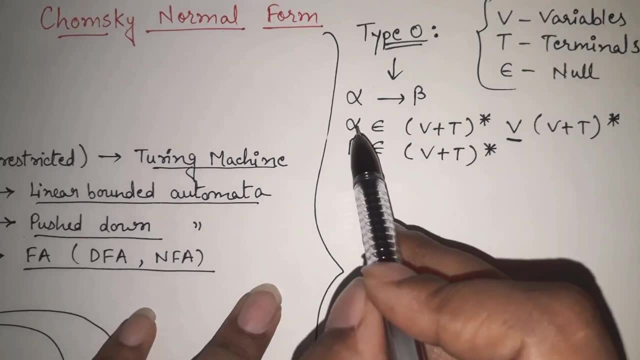 null in the beginning, at the end also, but in middle we have written v. that means what beta can have: anything, any variable or any terminal or null. So what is beta? beta can be anything, either variable or terminal or null. but the condition about alpha is alpha. 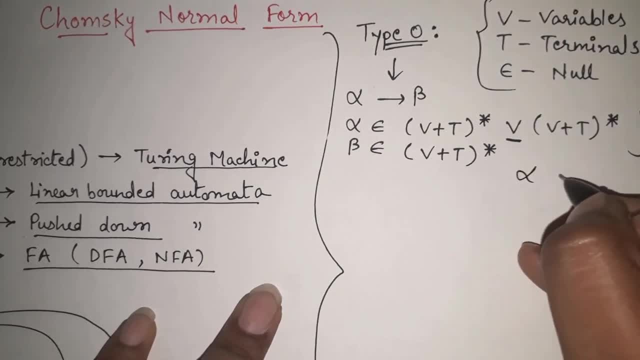 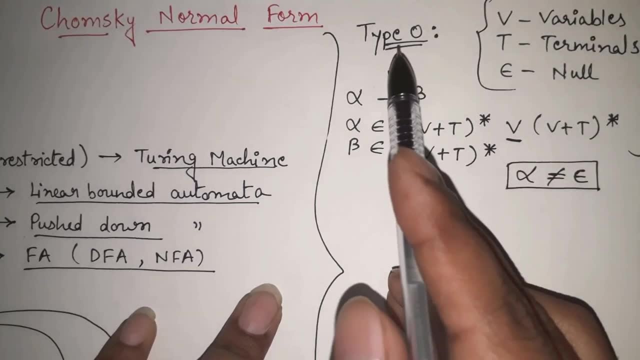 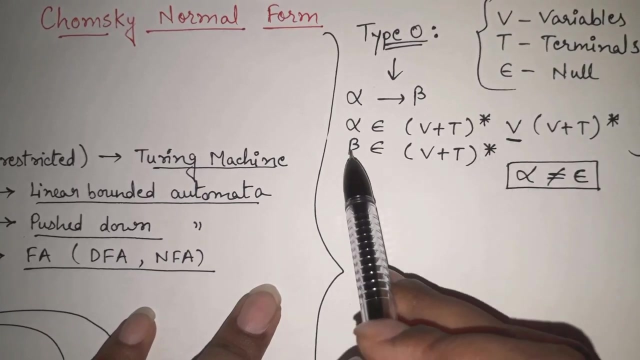 the condition about alpha is that our alpha in this case cannot be null. the only condition or the only restriction in case of type 0 is that alpha cannot be null. other than that means what alpha must be having at least one variable, and beta can be anything either variable. 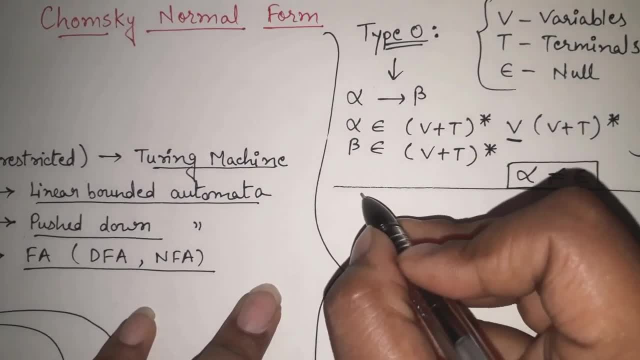 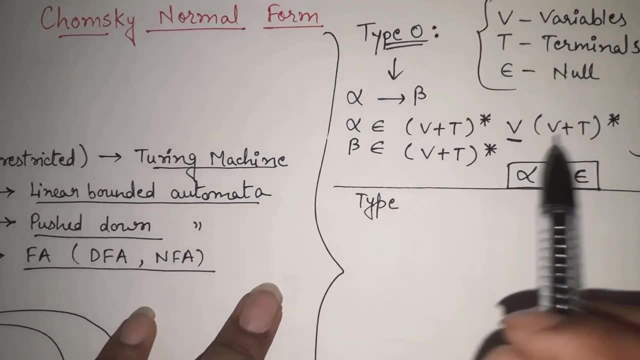 or terminal or null. Fine, Okay, So if I talk about type 1, so the only restriction in type 0 is alpha cannot be null other. all things are alright. Now if I talk about type 1, then type 1 is what this type 0- we have talked about that. 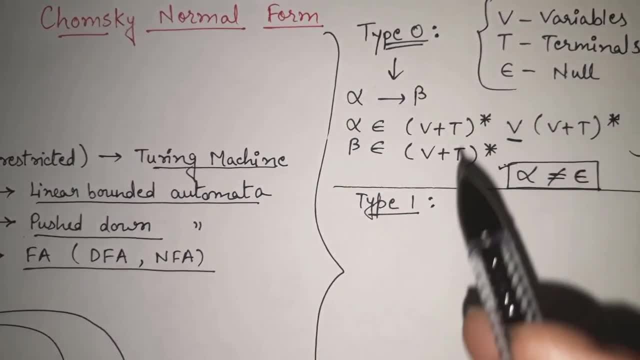 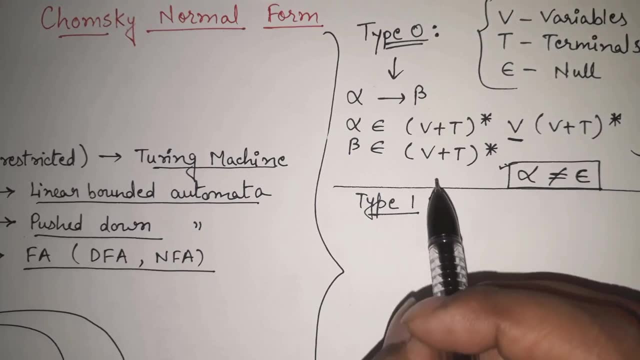 is unrestricted grammar, having only one restriction. this Now, type 1, is context sensitive language or context sensitive grammar in context C, as I have shown you, the relation. Type 1 may not be null. Type 2 may not be null. Type 2 will be null. 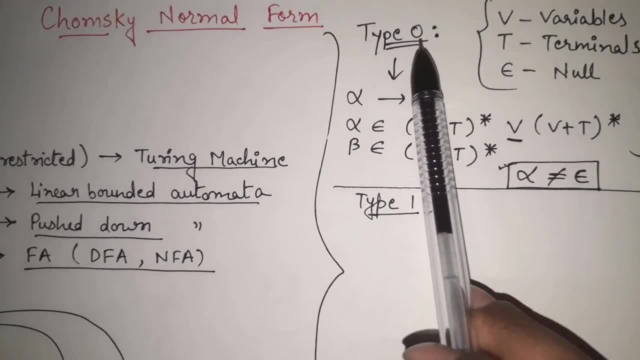 But type 1 and type 2 will be null. So I have already mentioned in SWOT, any restriction that is having that is present in type 0 will be present, will be automatically present in type 1, type 2, type 3 also. fine, because as we 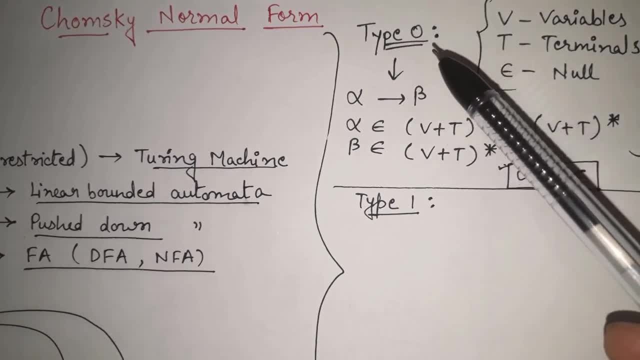 know, type 0 is unrestricted grammar. but if any condition is there or any restriction is there, that is present in case of this, that is present in case of unrestricted grammar also. So it will by default be in type 1, type 2, type 3 also. fine. 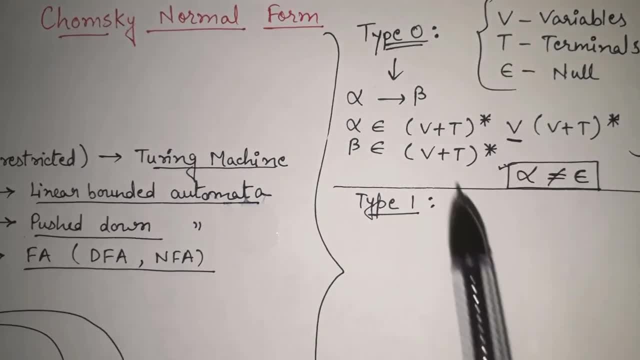 So we have already seen that type 0 is having restriction, that alpha cannot be null. So this condition is valid for type 1, type 2 and type 3 also. So apart from this restriction, the another restriction in case of type 1 is if we are having alpha gives beta. So the condition: 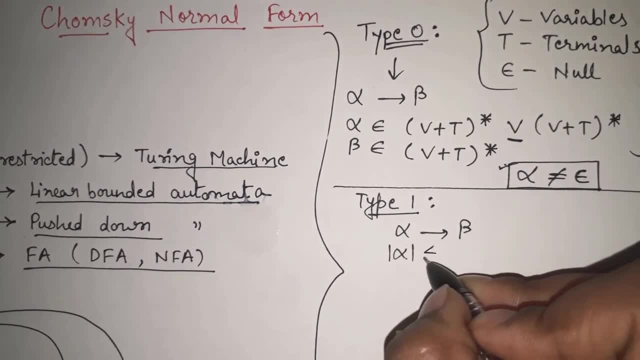 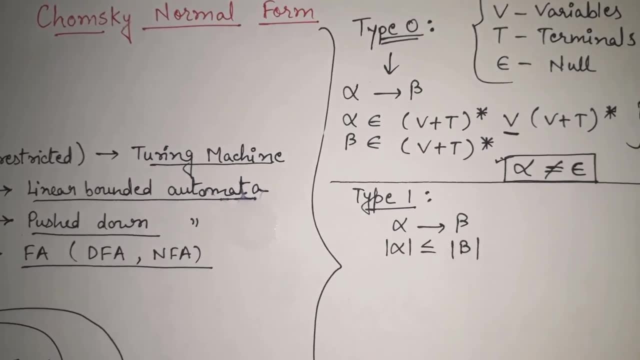 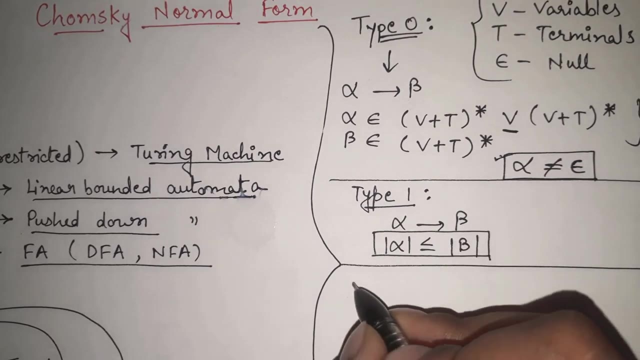 in type 1 is: the length of alpha must be less than or equal to the length of beta. That's it. This is the only condition in type 1 apart from this condition. Fine, So let me keep it in a box. So that's all about type 1.. Now, if I talk about type 2- and type 2 means what? context? free language. 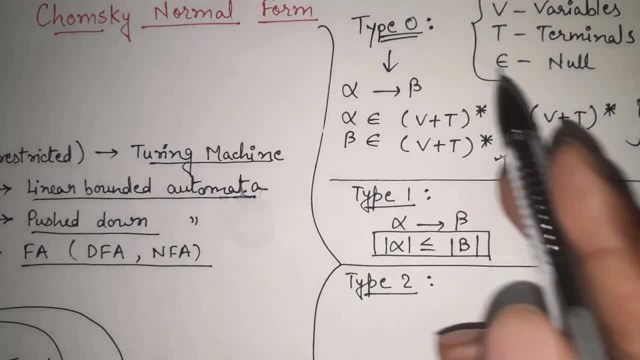 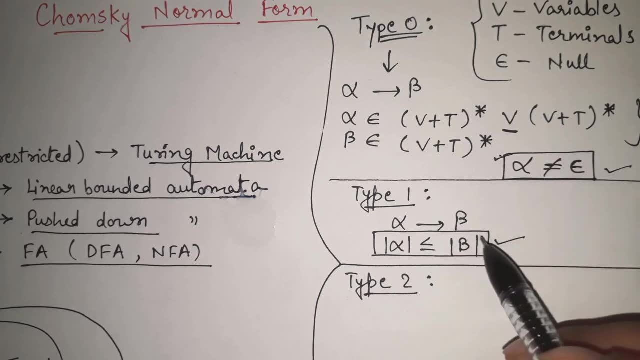 right. So what is the condition in type 2?? The condition that is present in type 0 and the condition that is present in type 1. these two will always be present in type 2.. So these two restrictions are already there. Apart from these restrictions, the third restriction of type 2 is: 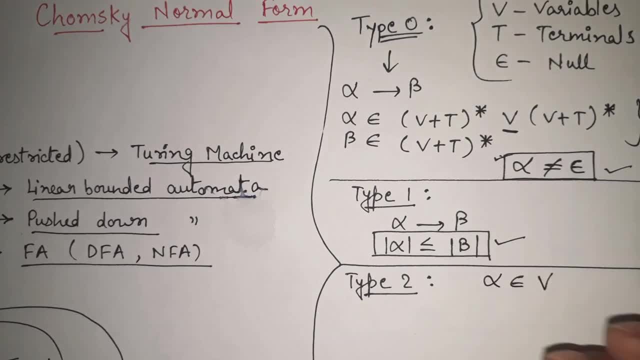 alpha will contain only one variable. Like in these two conditions what we have seen, Alpha can contain variable or terminal or mixture of variable and terminal. But in case of type 2, alpha will contain only variable and beta can contain either variables or terminals or null. 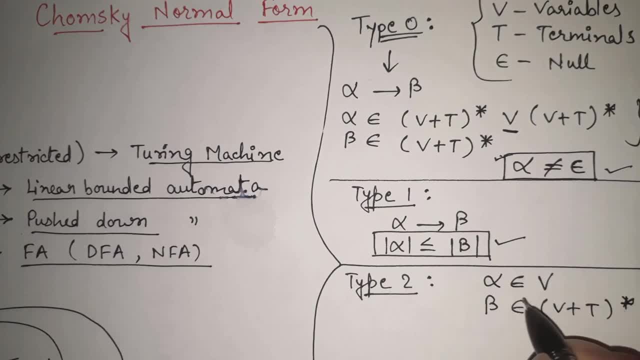 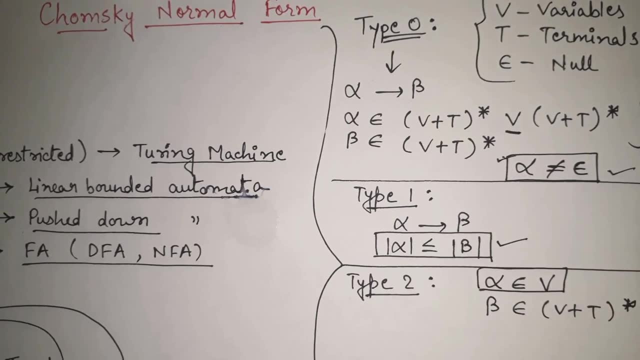 Means. there is no restrictions on beta, Fine, But there is your restriction on alpha. that alpha will contain only variable. So this is the condition in case of type 2.. Fine, Now we will talk about the last type, that is, type 3.. 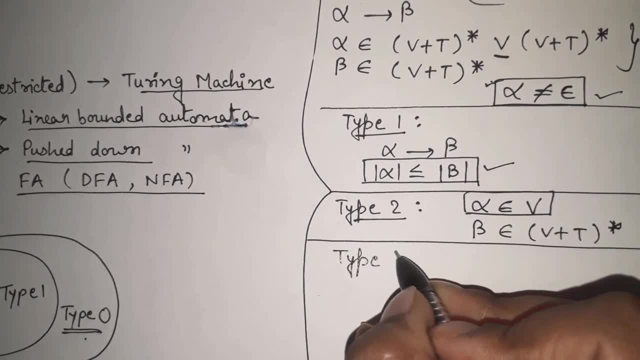 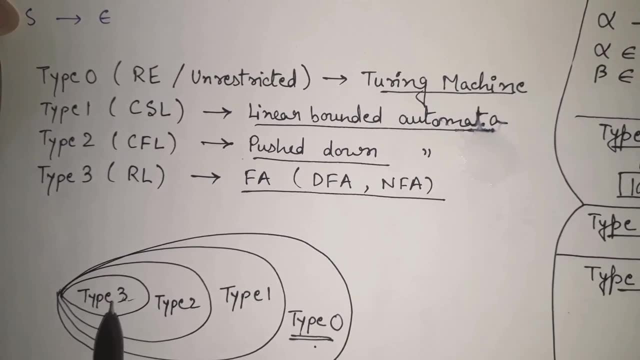 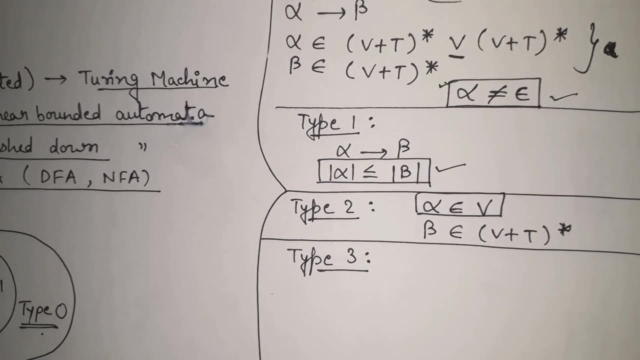 Type 3.. Type 3 is what Regular grammar And we can say that type 3, according to our this hierarchy, we can say that type 3 is our most restricted grammar, So as the name itself indicates regular or most restricted grammar. So like we have seen that in type 0, one restriction is there: Type 1. 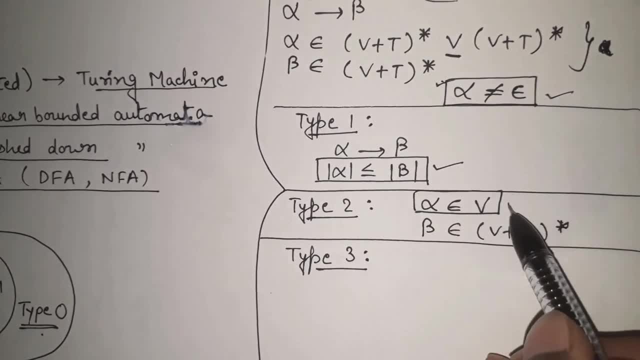 one special restriction is there, Type 2, one special restriction is there. So these restrictions, obviously they will be present in type 3.. But apart from these two conditions, what we have seen, apart from this, in type 3, we are having only two special cases and that grammar that will be present. 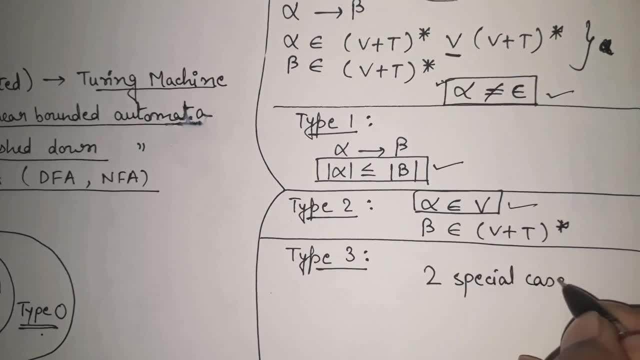 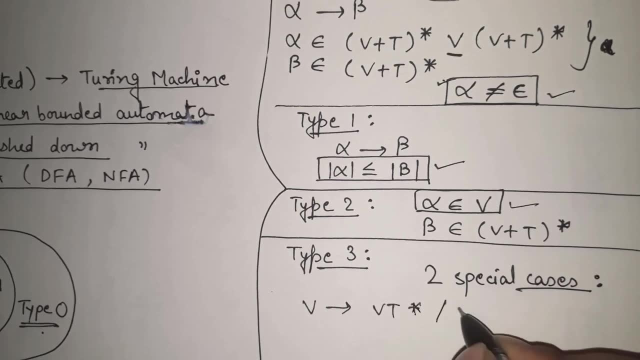 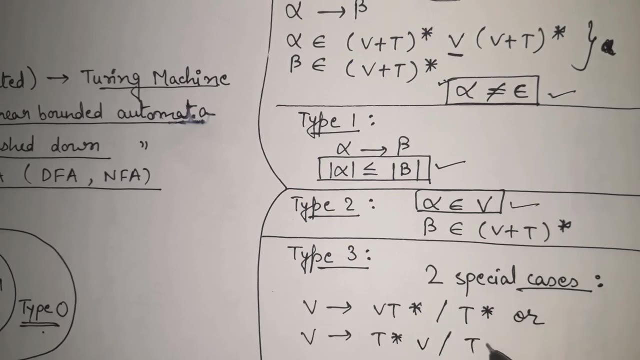 in type 3. the type 3 grammar will be of any of these two cases only. So the cases are that we can give v t star or t star. This is the one case. or our v can give t star, v or t star. So these are the. 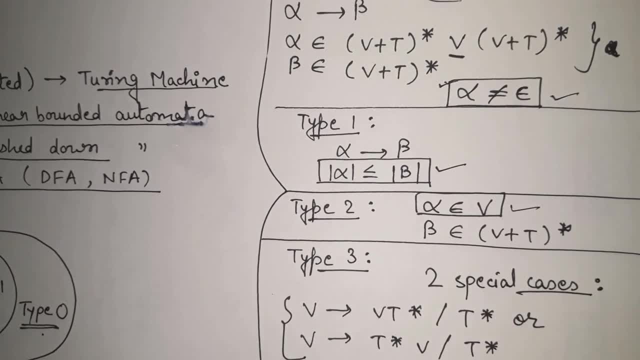 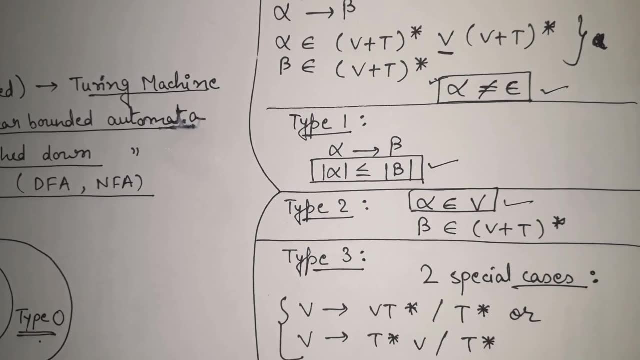 two forms out of these two forms. if my grammar is taking one of these forms, then only then I can say that my grammar is type 3 grammar. Fine, So these are the main conditions: 1,, 2,, 3 and this. These are: 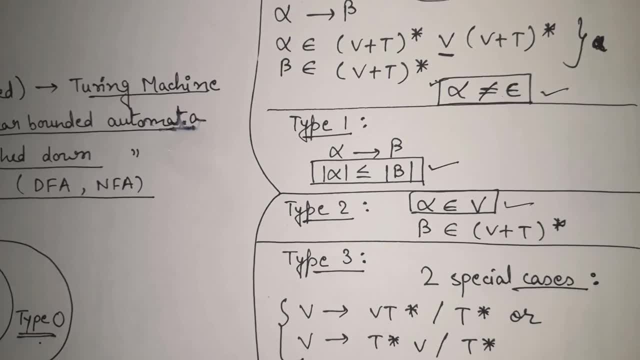 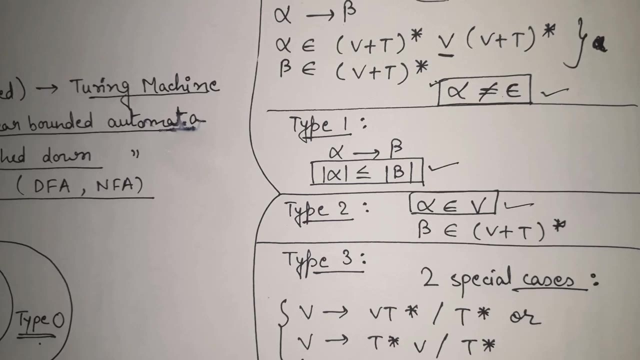 the main conditions that you should remember in order to know that, whether your grammar is that, in which category your grammar belongs to, Fine. So this is all about grammar that we should know. Now, in my next video, I will take some examples and I will show you that how to categorize our grammar in any one of these forms and how to